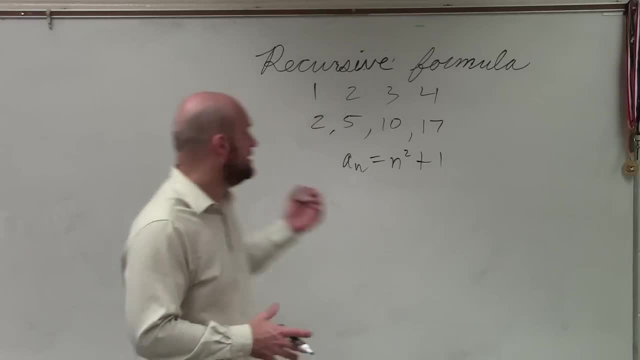 Okay, So the recursive formula is going to have a different way here. the way to find our rule, or the way to find the next value, is to identify the rule, right, And then, once we know the formula, we can find out any number in the system, correct, Right? If I said, what is a sub 12, we just put in 12 in for there. Does that make sense? 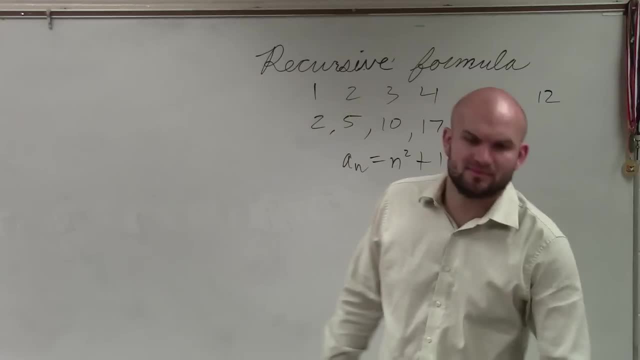 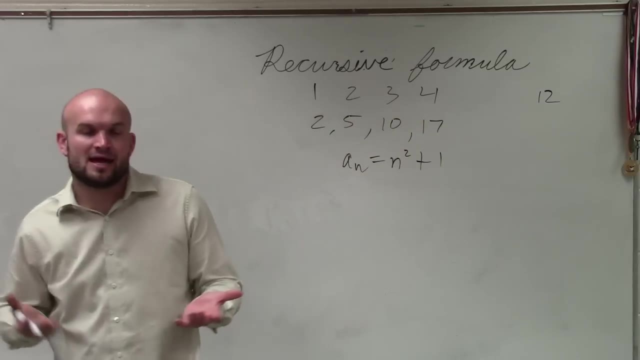 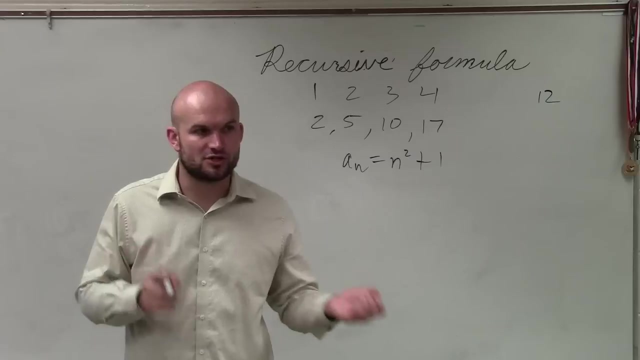 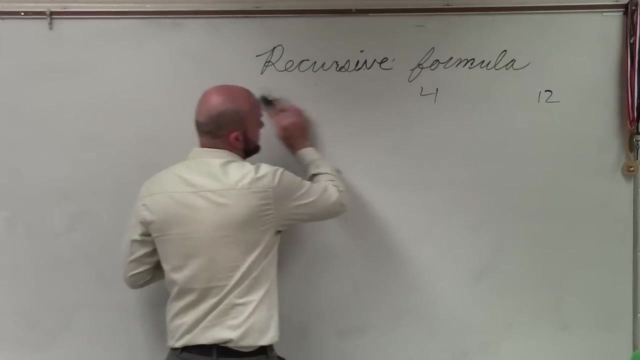 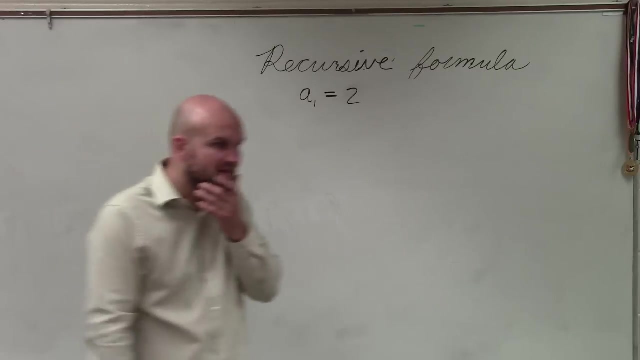 Yeah, Right Now, Colby, I'm just going to have you actually move up to one of these seats for you. So now, what we need to, now what we're going to talk about, is the recursive formula. Okay, And the special thing about the recursive formula is it's based off of the previous term. All right, So let's look at this in a recursive formula format. Let's say, I give you the first term in the sequence, which we'll call a sub 1, first term equals 5.. And let's do make it simple, Let's do 2.. All right, 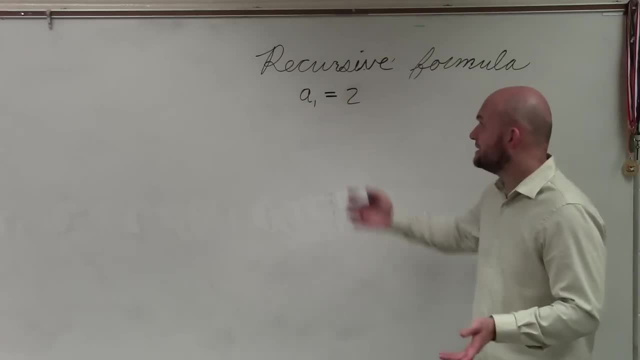 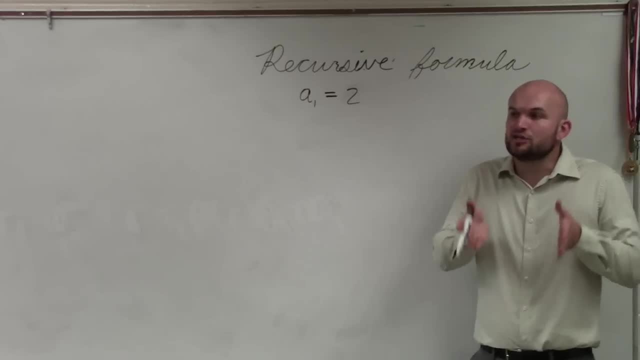 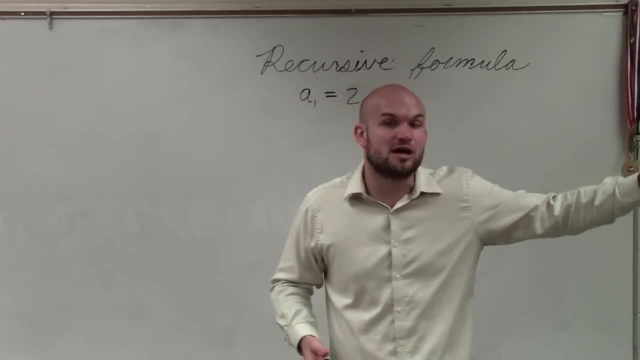 All right. So it's not just the turn, It's not just a formula to, if I had to go from every number to it's term, It's how do you find the next turn. So we can label that recursant formula. 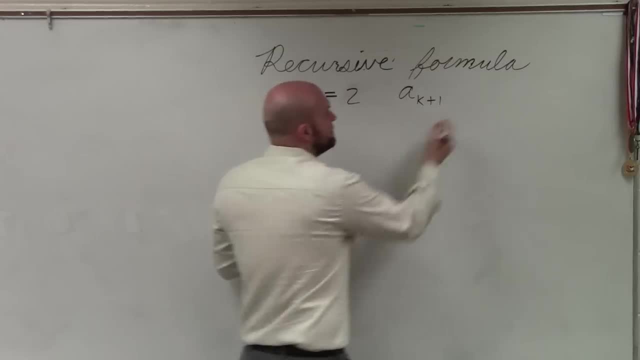 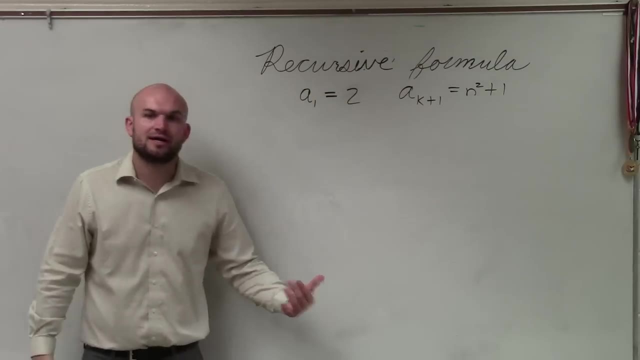 Pass a of K plus one and let's same. Okay, So what we're going to use for the recursive formula is: now we're going to find the next five terms. It's not a simple, you know, so when we plug them in, 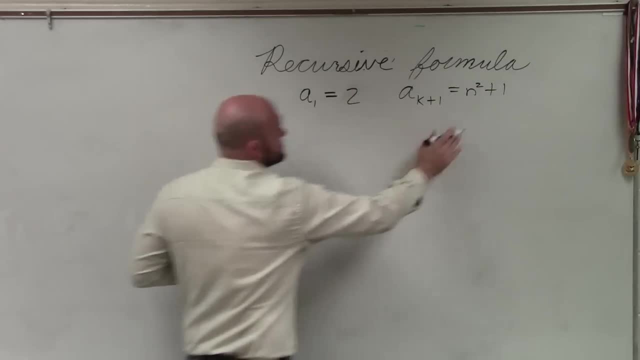 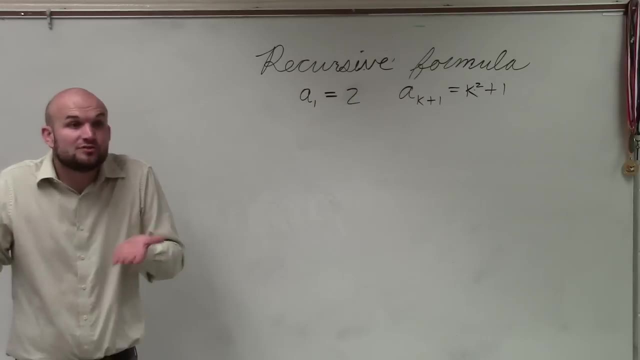 just like we did before. let's plug the 1 in for the k. I could use n's again if I wanted to. You could use l's. You could use p's. We're using k for the recursive formula in this case, okay. 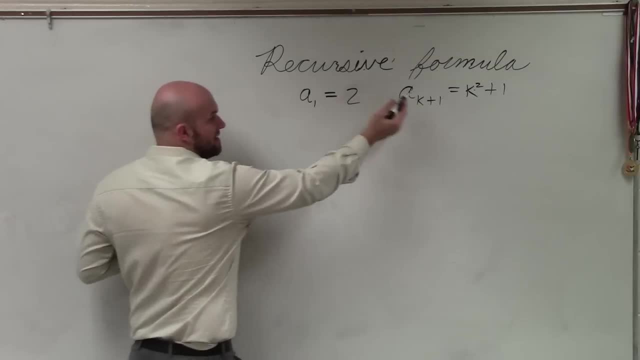 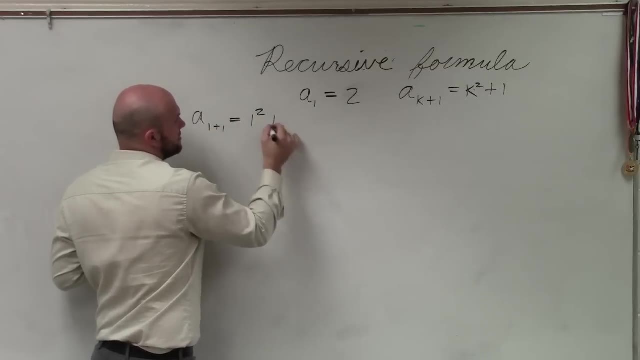 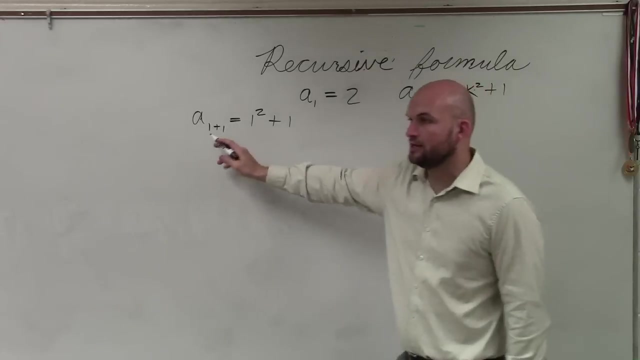 So if I was going to plug in 1 into my formula, I'd have: ace of 1 plus 1 equals 1 squared plus 1.. Would everybody agree? Sure, Yes, Ace of 1 plus 1 is ace of 2, right. 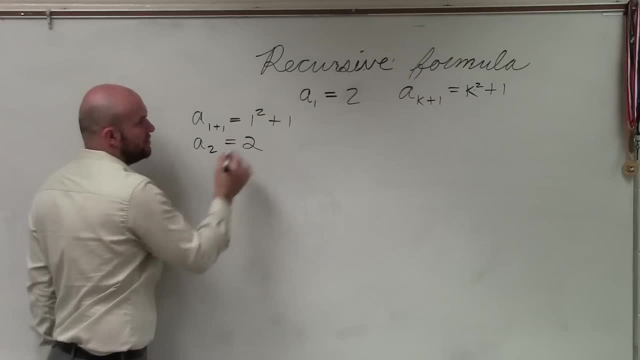 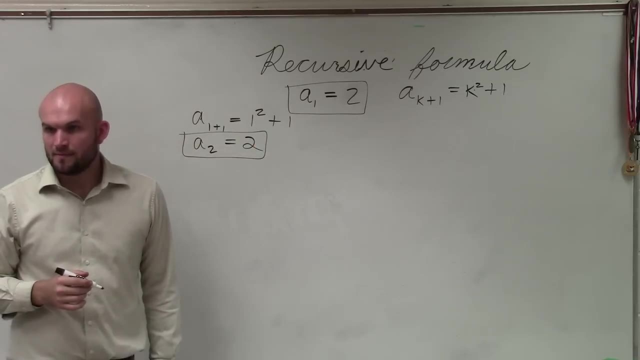 Equals: 1 squared is 1.. 1 plus 1 is 2.. Do you guys now see how I just found the next number in the sequence? Yeah, Did you guys see that? So now I use the recursive formula again to find a of 3.. 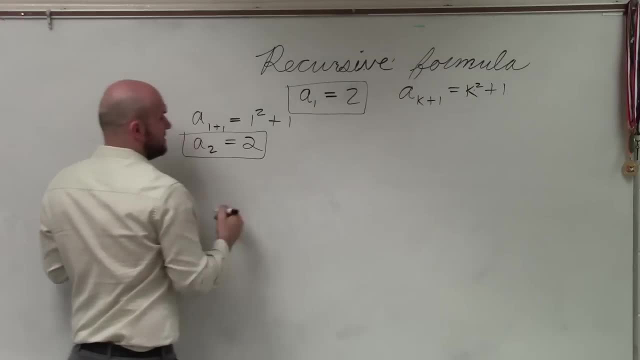 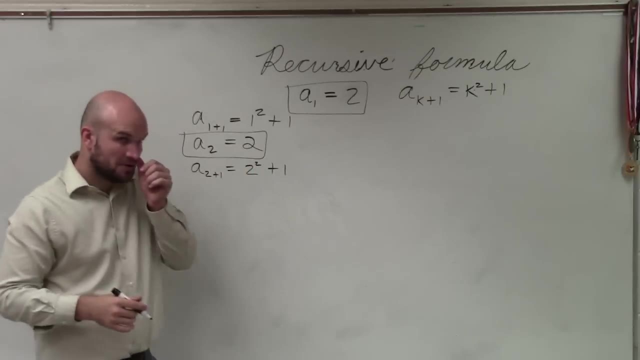 What you do is again you put in your 2 in for your k. So I have ace of 2 plus 1 equals 2 squared plus 1.. Ace of 2 plus 1 is going to be ace of 3, which is my next term. 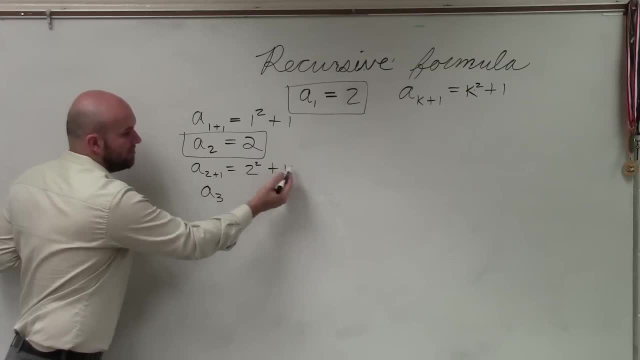 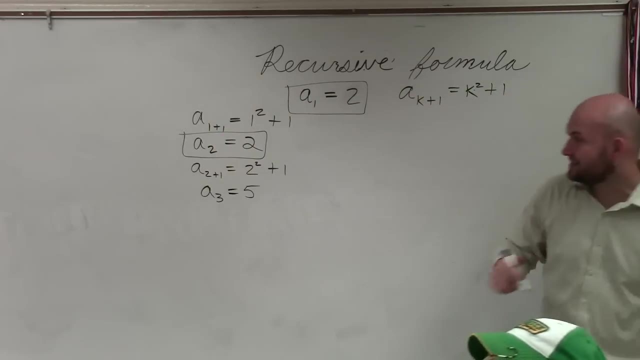 2 squared is 4.. 4 plus 1 is 5.. All right, And then do you guys kind of see the pattern now Do you guys see how we're going to get ace of 4?? Yes Question: Does that mean that ace of 2 equals 2?? 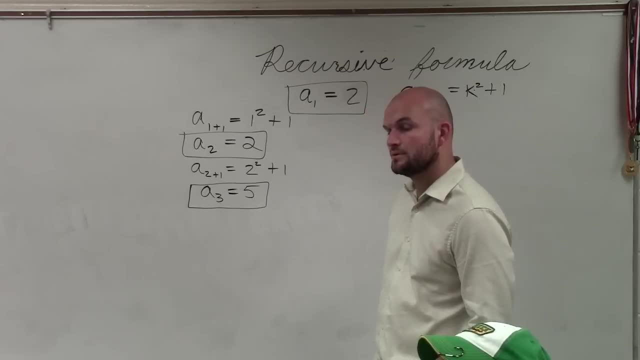 Yes, that's the value for ace of 2.. So is ace of 1 exactly that. That's like the starting. Yeah, it's the same thing. That's your starting point, But what I'm saying is to go to the next term in the recursive formula. 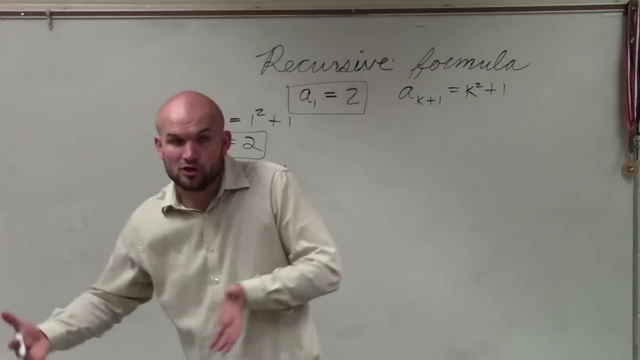 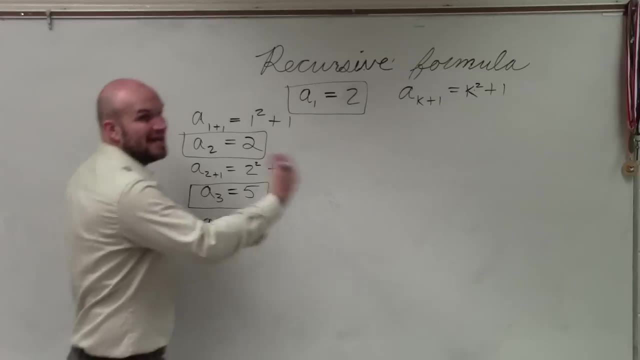 it's based off of the pattern. So if I'm going to find ace of 2, I'm going to have to use ace of 1.. So to find ace of 2, we have to use ace of 1.. To find ace of 4, to find ace of 4, we have to use ace of 3.. 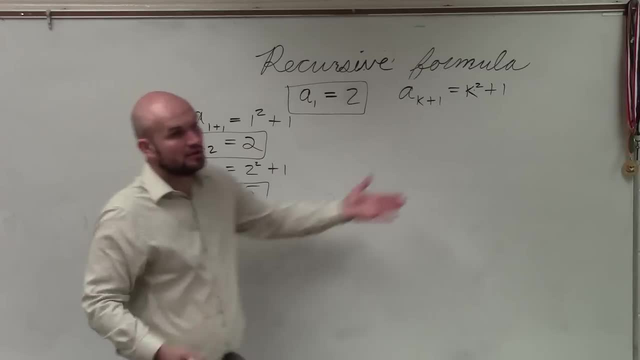 So what I'm simply going to do is plug in the value for my ace of 3.. That's the formula, Okay, Oh, and actually I wrote yeah, so your k. So my ace of 4 is simply just going to be my previous term, which is ace of 3.. 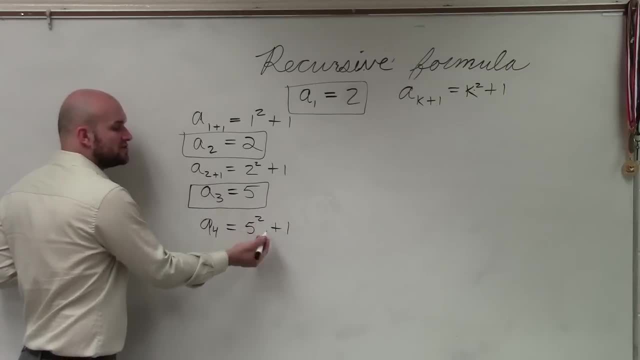 And for that it would be 5 squared plus 1.. 5 squared is 25.. So 25 plus 1 is 26.. Now I'm not going to do the fifth term because obviously 26 squared is going to be a pretty large number and we can just go through it. 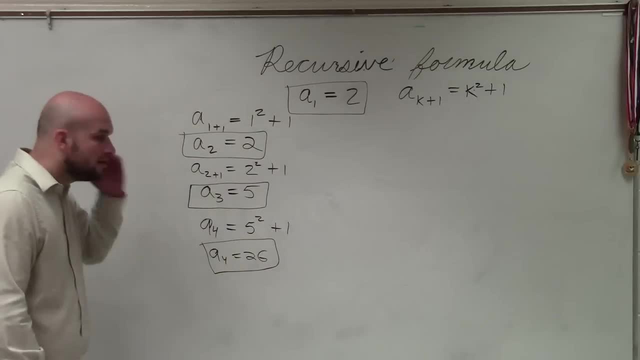 Yes, Why do you use 5? So to find ace of 1, right that was given to us To find ace of 2,. what did I do? I didn't plug in the first number. Crap, I did that wrong. 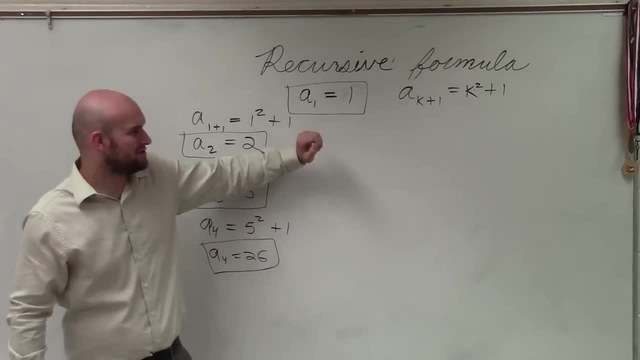 That's fine. Oh Yeah, Thank you. Sorry about that. Let's just change this so I don't have to change my work. Well, let me make this clear: To find ace of 2, to find ace of 2, you plug in ace of 1, right in 4.. 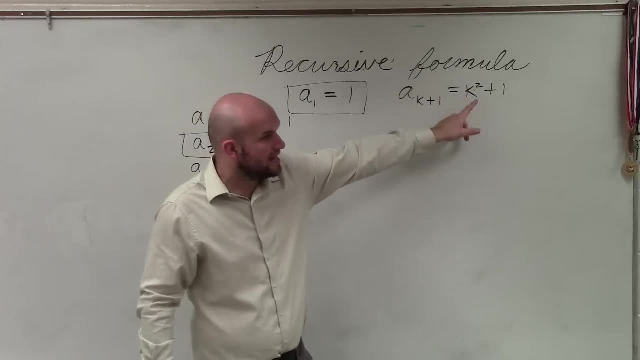 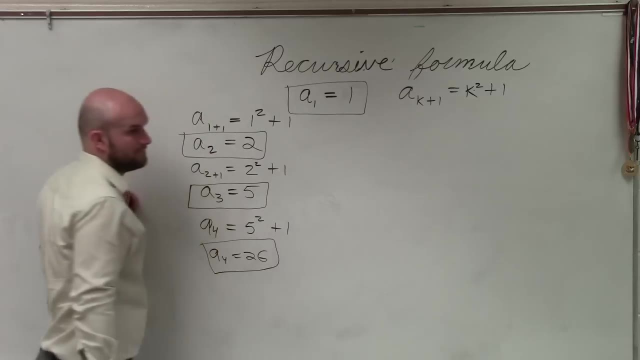 To find your ace of 1, you plug that 1 in for your k. So you're pretty much. what you're doing is you're plugging in the previous value into your formula. Oh, so you're just using the right number. 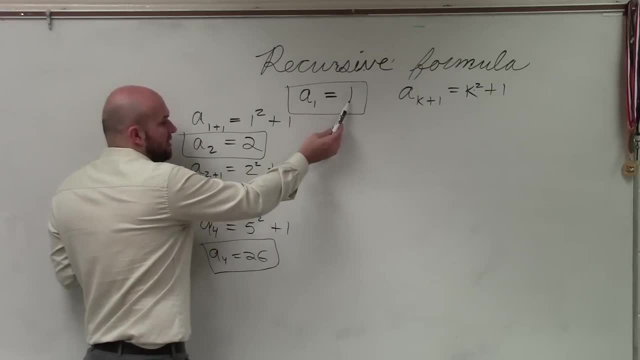 You're using the previous number. So here I have: ace of 1 is 1.. Oh, I see. So what I did is I put 1 in for k To find ace of 3, 2 was ace of 2.. 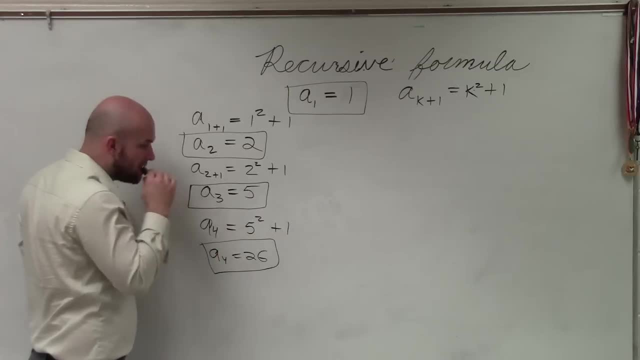 I plug in ace of 2 into the formula. Yeah for ace of. yeah for that one, you did 3 and then 5.. Shouldn't it be 5 plus 1? Ace of 5.. So so, ace to find ace of 3, I mean to find ace of 4,. 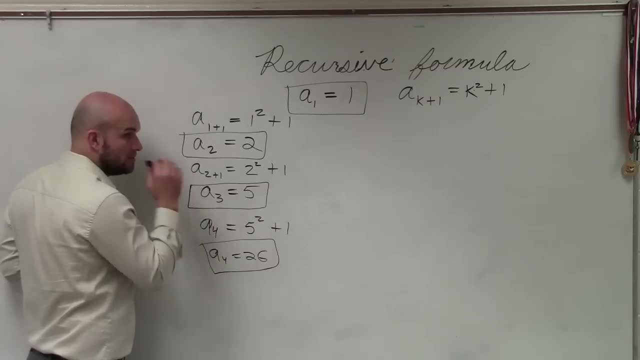 I plug in the previous term. But then why did you have a subscript? Because, like you, just ate sub 2, and then ace sub 2 plus 1.. Yeah, Did you use a subscript, Or did you use the 2 from up there? 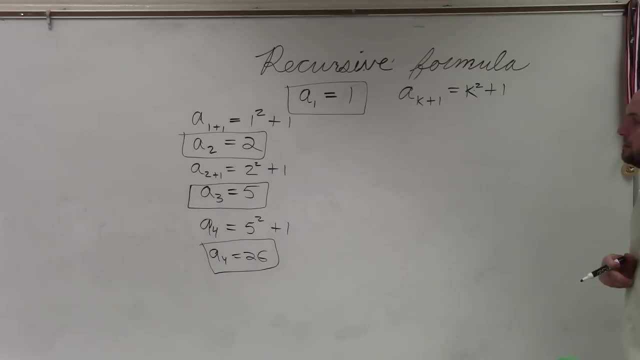 1. Do you just? It's just, I don't know, I'm going to put 5 on it. I'm going to put, you know, oh, come on, You have ace of 3, right, and then you get 5's right. 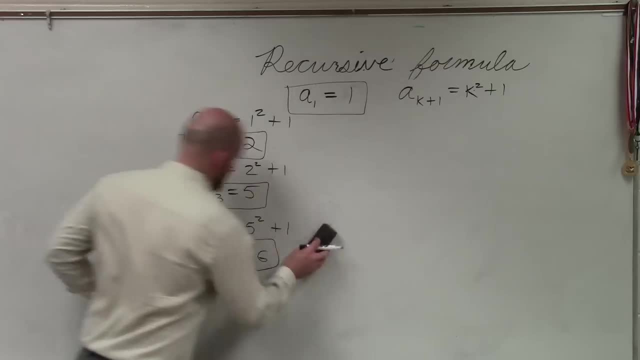 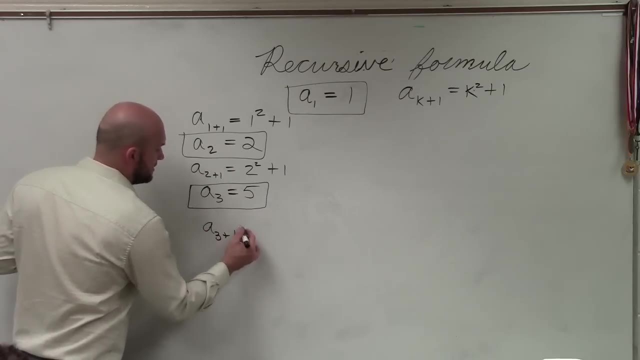 Yeah, but shouldn't it be ace of 5 plus 1?? No, no, it's, you know. so we plug in ace of 3 into our formula. Ace of 3 plus 1 equals or ace of 3, what is ace of 3 equal?